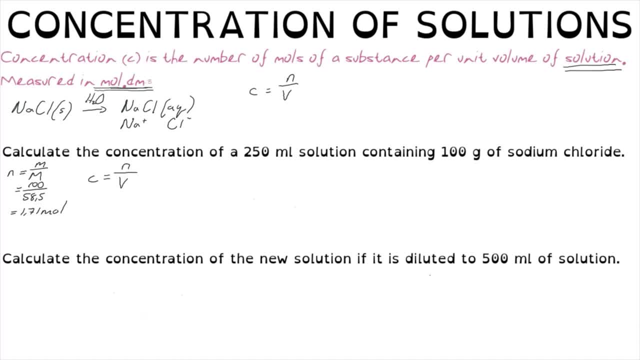 of the sodium chloride solution is equal to the number of moles divided by the volume. But just a note on volumes. in chemistry the preferred volume or the preferred unit for volume is cubic decimetres, which is a cube that is 10 centimetres by 10 centimetres, by. 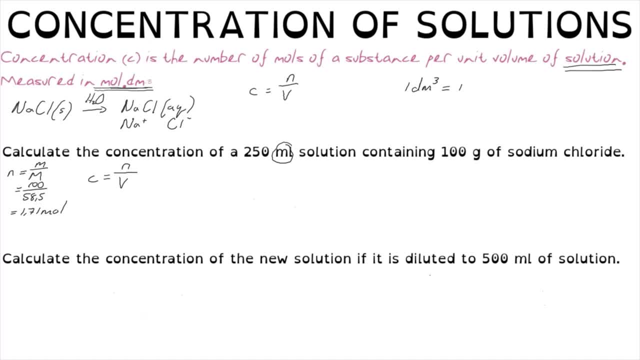 10 centimetres. A cubic decimetre is exactly the same as one litre of solution, which is also, as we know, the same as 1000 millilitres of solution, or 1000 cubic centimetres of solution. 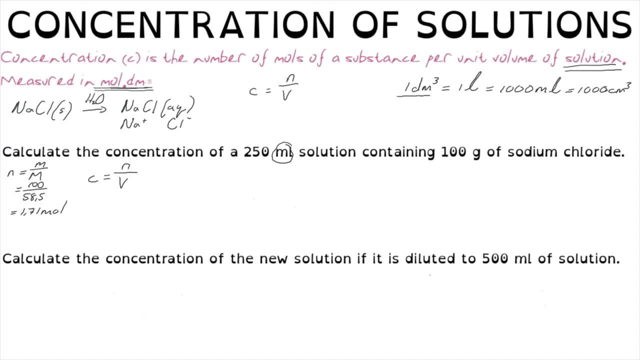 So no matter what volume we are given, we would always convert it into cubic decimetres. In this case, we have been given a volume of 250 millilitres and we say 250 millilitres divided by 1000 to find that it has a volume of 0.25 cubic decimetres. 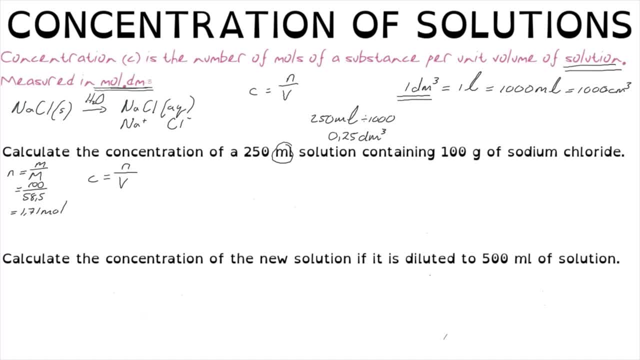 And so we can now say that the concentration of the solution is our number of moles of sodium chloride in the total volume of the solution, which is 0.25 cubic decimetres, which is therefore a concentration of 6.84 moles per cubic decimetre. 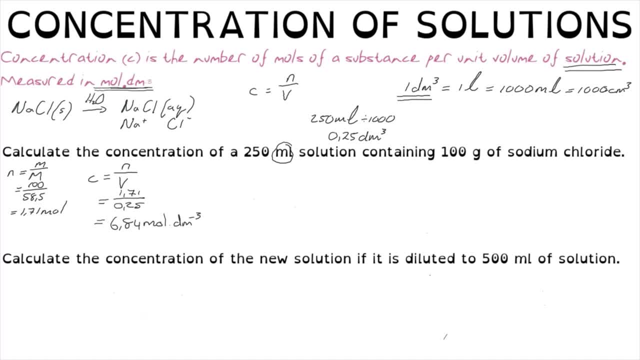 What that tells us is that if we were to have one litre or one cubic decimetre of the solution, that would contain 6.84 moles of solution. Clearly, we only have a quarter of a litre, 0.25 cubic decimetres and therefore only 1.71 moles of solution. It's important to 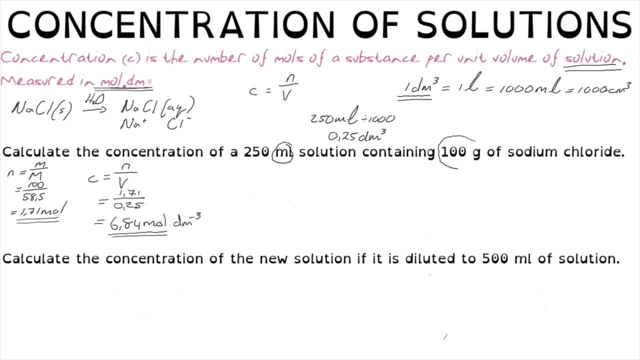 note here that when we dissolve one substance in an atom, we dissolve another one in an another. so 100 grams of sodium chloride in another. That does not affect the volume. The reason for that is because that substance will ionise or dissociate and form a part. 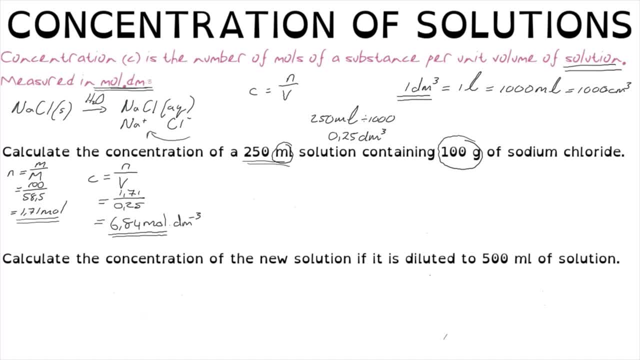 of the solution. It does not increase the volume of the solution. Another follow-on question to this that's quite common is where we are asked to either dilute or to calculate the concentration of a diluted solution. A common question here would read: calculate the concentration of the new solution. 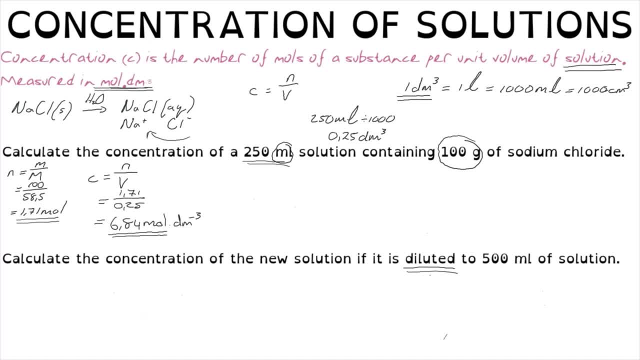 or the diluted solution, if it is diluted, to 500 millilitres of solution. What that tells us is that the volume of the solution is taken from 250 millilitres to 500 millilitres, which means that we're adding 250 millilitres of water. It is important here that when they 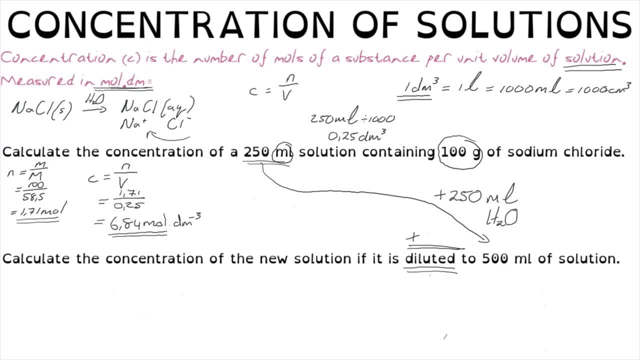 use the word diluted. that means that there is no further sodium chloride added. We are only increasing the volume of the solution Now, since there is no sodium chloride added. we are only increasing the volume of the solution Now, since there is no sodium chloride added. 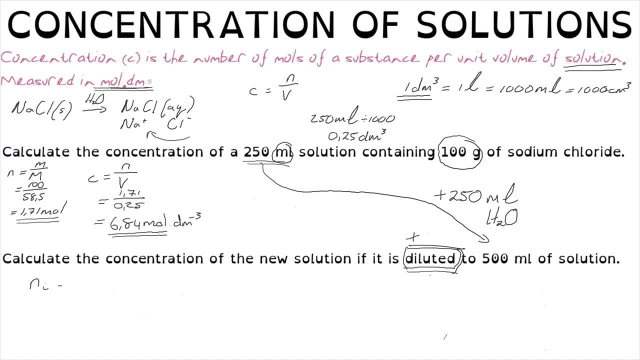 we can say that the initial number of moles of sodium chloride must be equal to the final number of moles, which means that the initial concentration multiplied by the initial volume must be equal, therefore, to the final concentration multiplied by the final volume, because, using this formula over 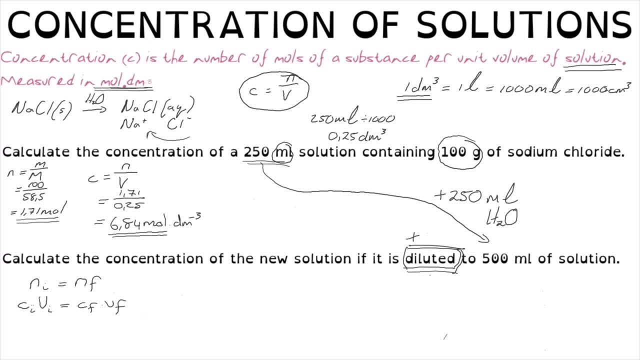 here the concentration is equal to number of moles of a volume and therefore the number of moles is equal to concentration times volume. so our initial concentration we've just worked out was 6.84 moles per cubic decimeter. the initial volume in cubic decimeter was 0.25. the final 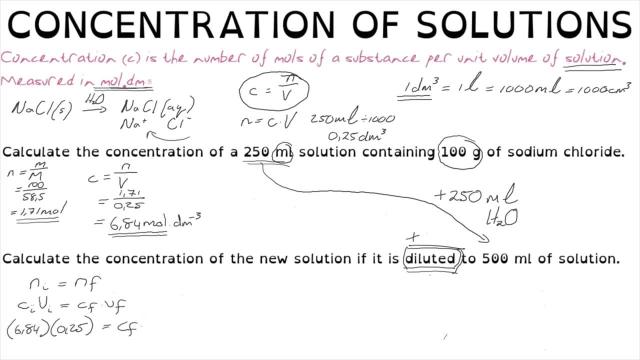 concentration is our unknown and the final volume? we've been told it's been diluted to 500 milliliters, so 0.5 cubic decimeters, which therefore tells us that the final concentration of this new diluted solution is 0.5 cubic decimeters. 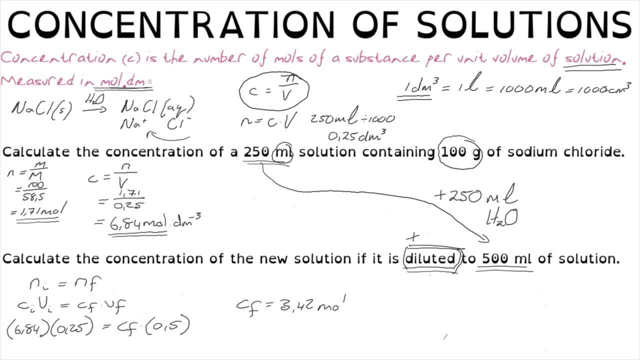 3.42 moles per cubic decimeter, which should make sense to us, because we have taken the same number of moles of sodium chloride and we've doubled the volume. so therefore we should have the concentration of the solution. so now, using the formula, concentration is equal to the number. 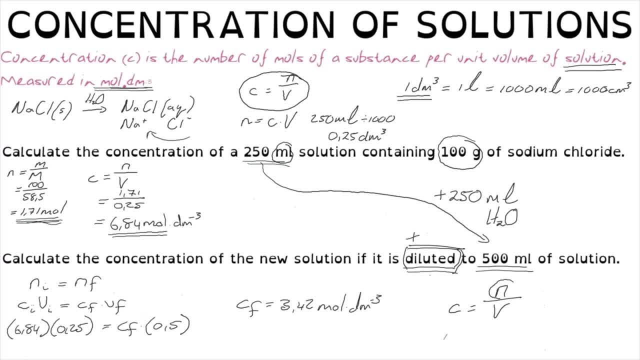 of moles over the volume. we can always calculate either the number of moles when we know the concentration and volume of a solution. or we can calculate the concentration when we know the number of moles and volume of a solution, or we can calculate the volume required if we know the 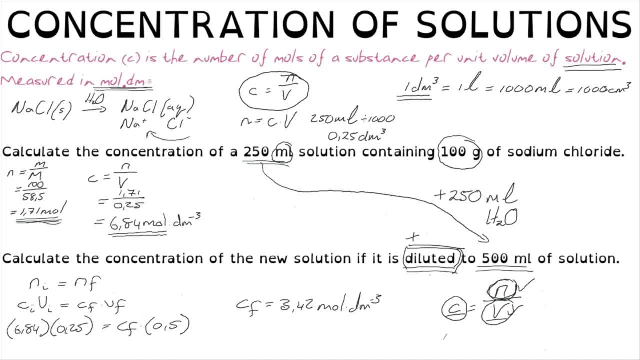 number of moles and concentration of a certain solution. you